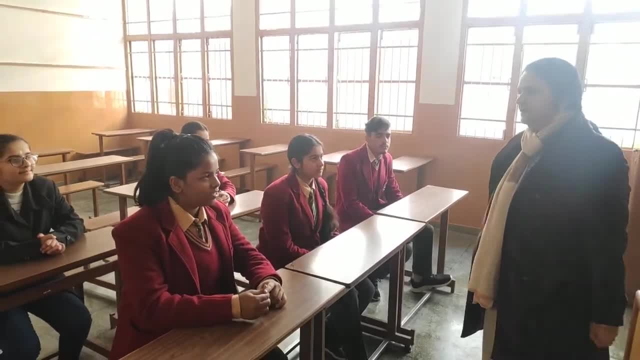 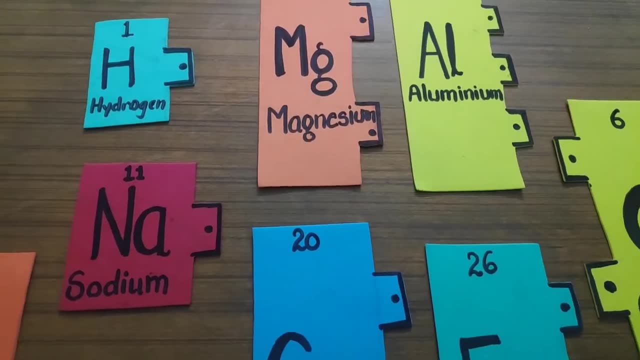 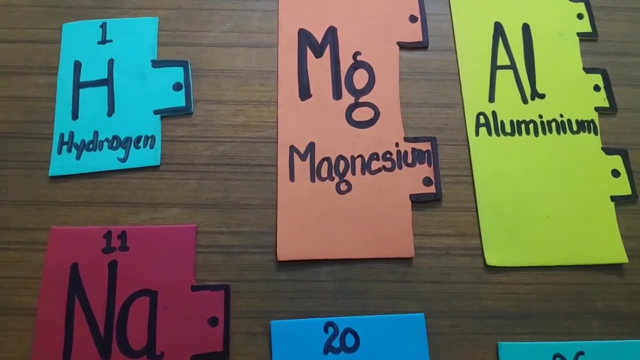 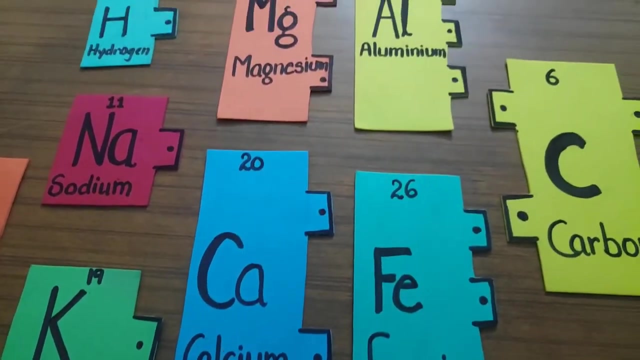 Many substances which we are using in our daily life. So let us start with this activity. As you can see, few cards are lying here and each card is representing one element, And I have written the name and the symbols of the elements, as you can see: H for hydrogen sodium, Na, potassium, K, etc. And what is specific in this game is that 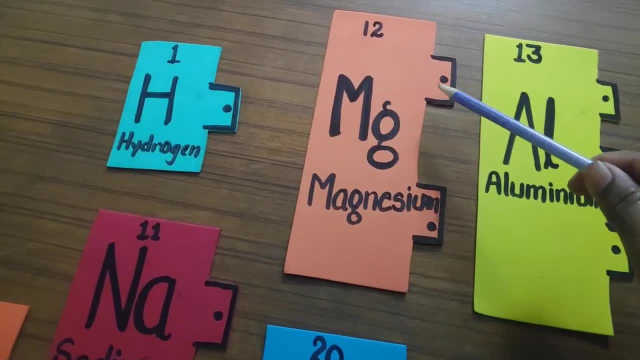 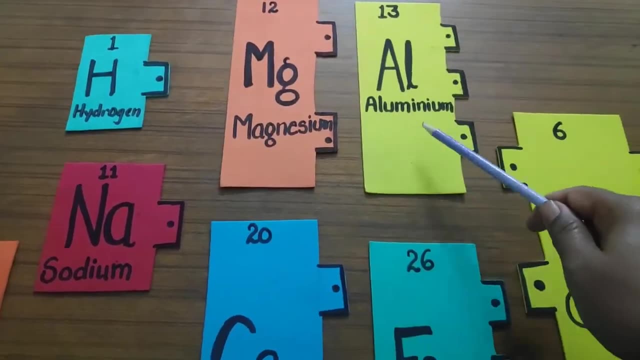 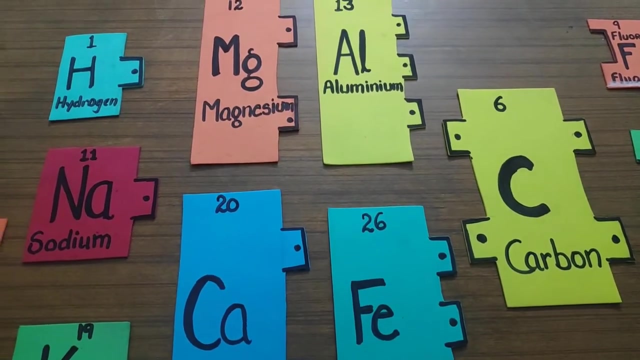 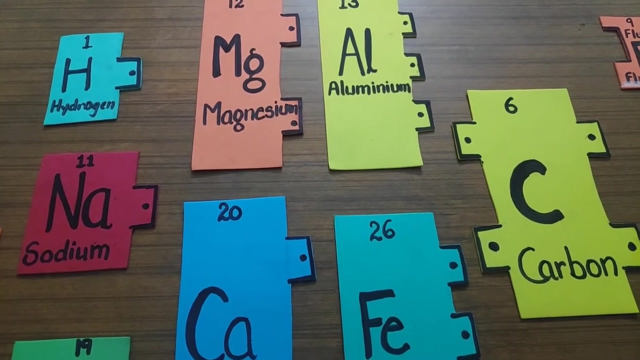 each card has a specific number of arms. For example, few cards you can see have one arm. These cards have two arms. These cards have three arms. This carbon has four arms. These arms actually represent the valency of elements. Valency, you know, na This is the combining capacity of an element. Means the number of chemical bonds which an element can form during 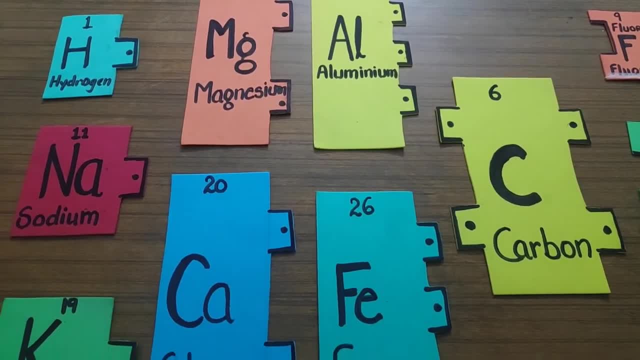 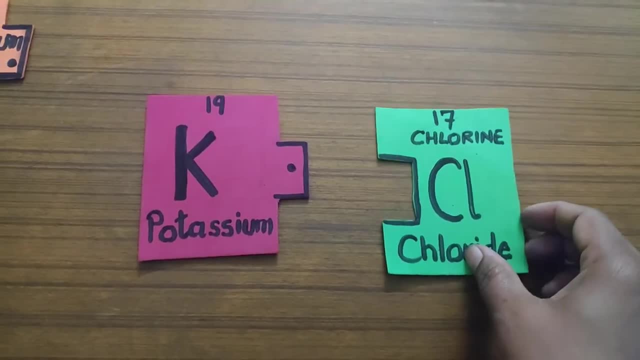 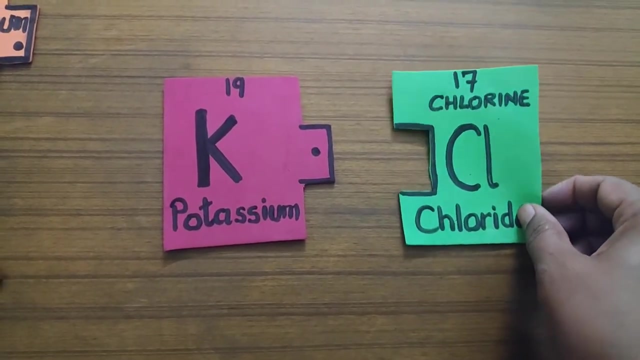 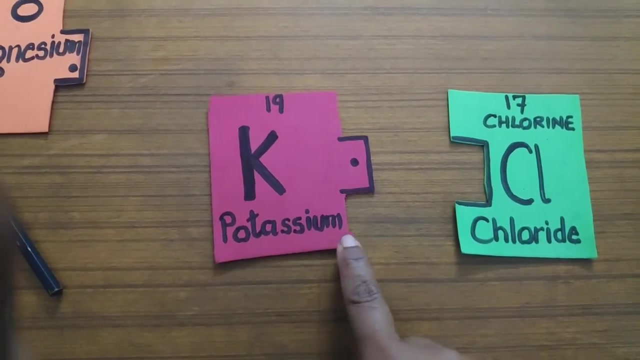 combination with other elements, So that represents the valency of each element. So in this way, these arms represent valency. And to start joining these cards to obtain chemical formula. So I have taken two cards here having one arm each And, as you can see, these arms are in different manner. Potassium has arm like this, which represents the electron losing tendency of potassium, And chlorine has arm. 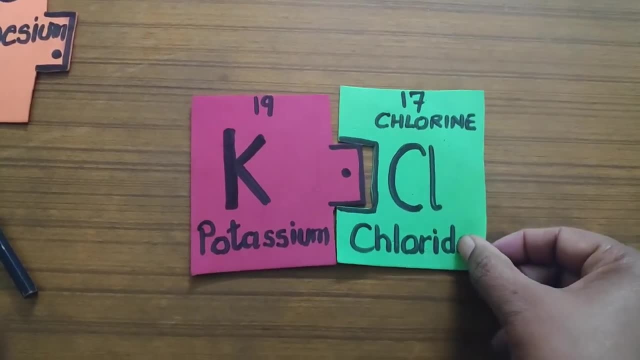 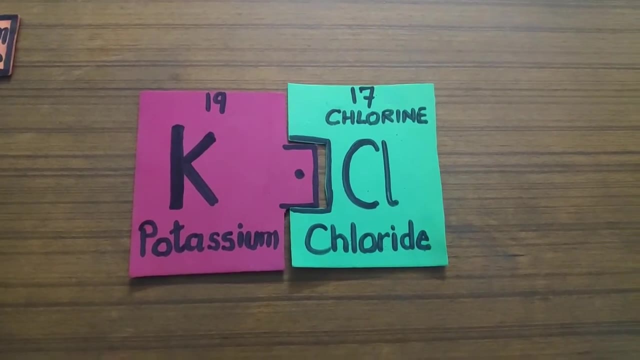 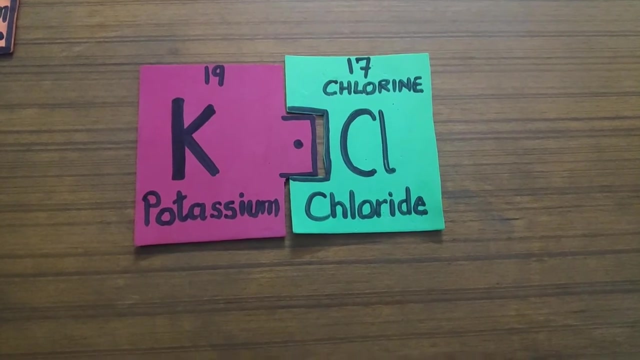 in this manner that during combination it gains the electron lost by potassium. so this is how the two different types of arms are shown by these cards and you can prepare variety of compounds by satisfying these arms, or you can say satisfying the valencies of elements. you can prepare variety of formula. so this: 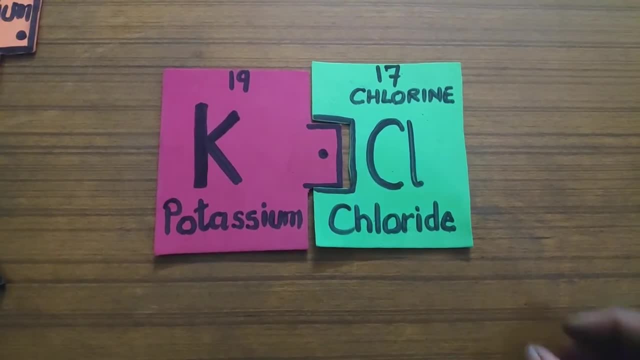 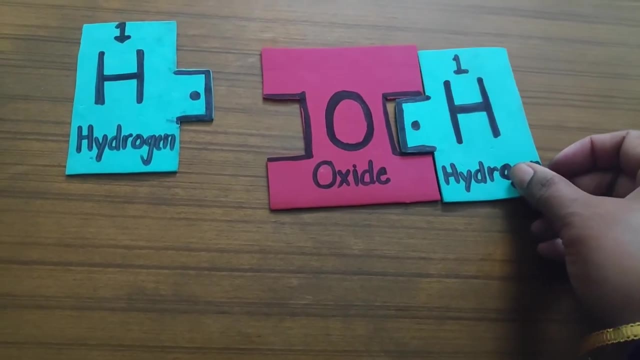 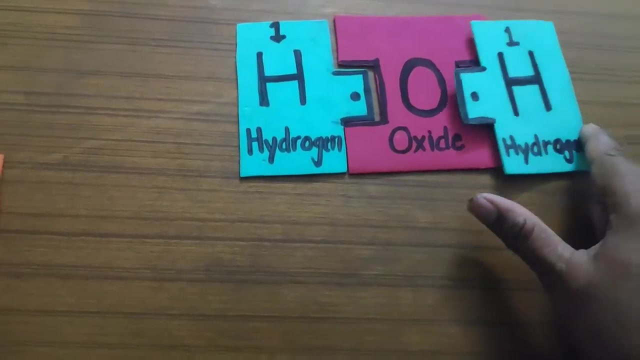 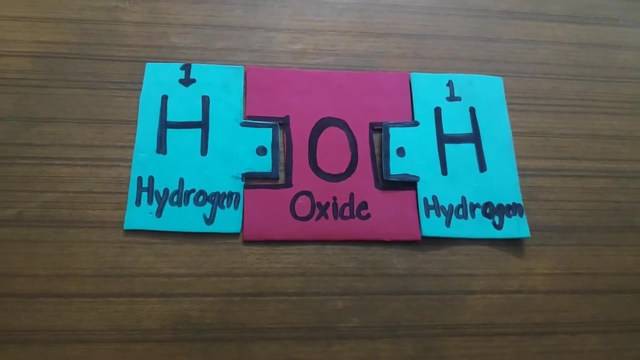 is potassium chloride, formula is KCl. now, now we can prepare the formula of water by using these cards of oxygen and hydrogen, as oxygen has two arms and hydrogen has one arm, so you can join oxygen and hydrogen atoms in this manner to form the formula of water as H2O, as two cards of hydrogen are combining with. 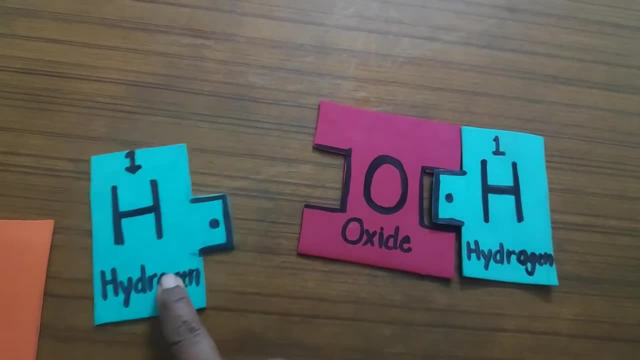 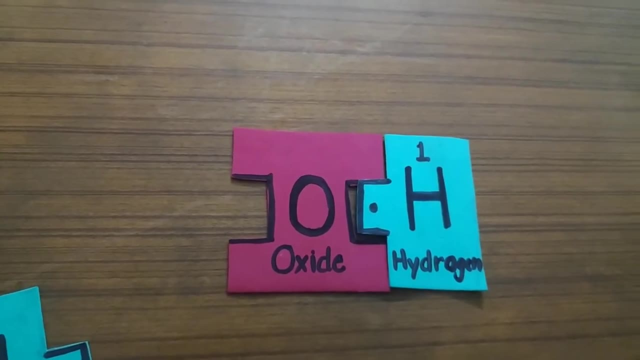 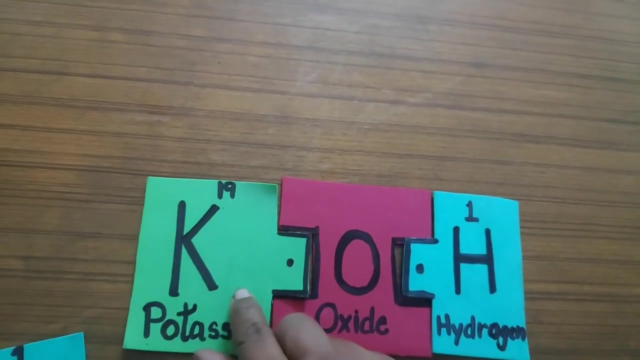 one card of oxygen. now suppose if we remove this card of hydrogen we get a species having one arm free, and this is known as hydroxide ion. now suppose if we add one card of potassium to this hydroxide ion, we obtain formula of potassium hydroxide. 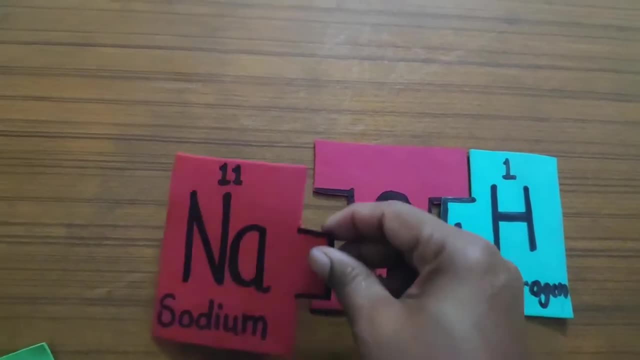 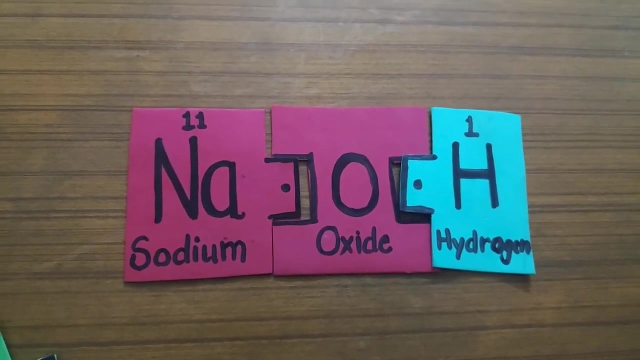 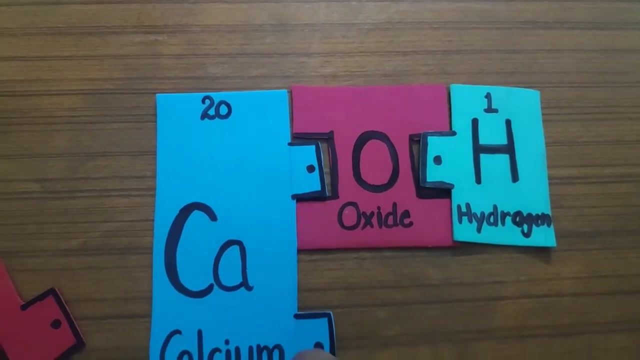 and if we replace this potassium with sodium atom, then we find the formula of sodium hydroxide, which is NaOH. now suppose, if we want to make high formula of hydroxide of calcium or magnesium, which have two arms, so we need to add one more hydroxide ion to this in. 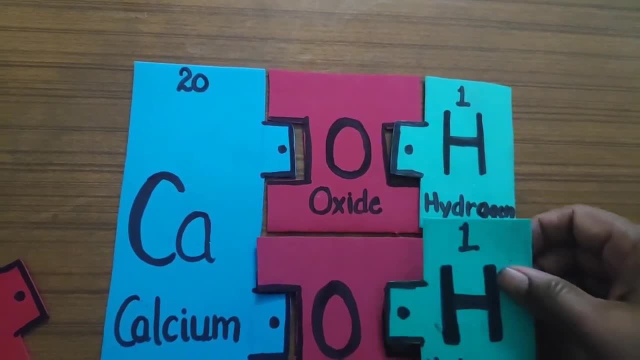 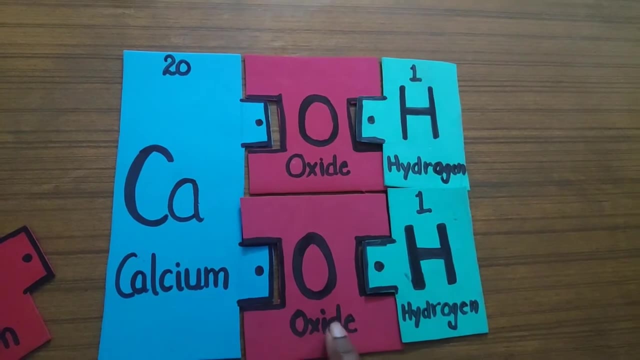 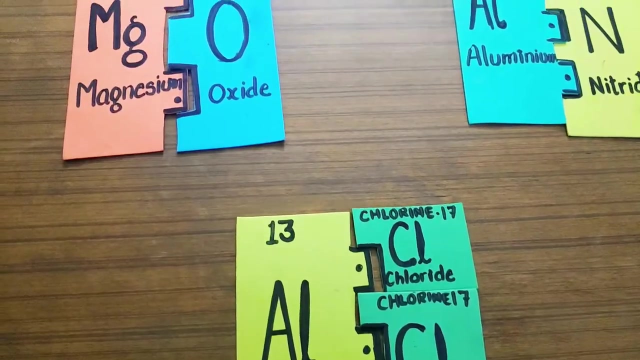 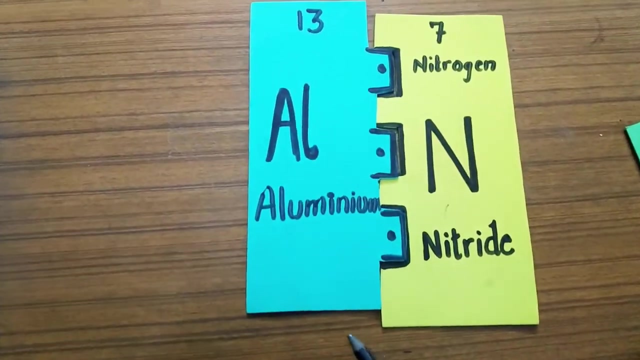 this manner, and here we can have the formula of calcium hydroxide as CaOH twice as twice O H ions are used here. okay, so various combinations are possible, like formula of magnesium oxide. we can obtain, like this, aluminum nitride. having both cards of three arms, we can join them in this manner and 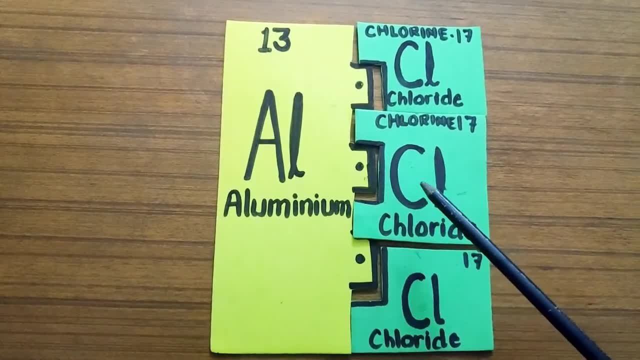 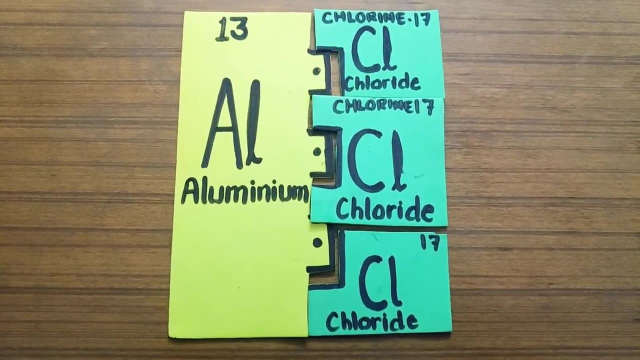 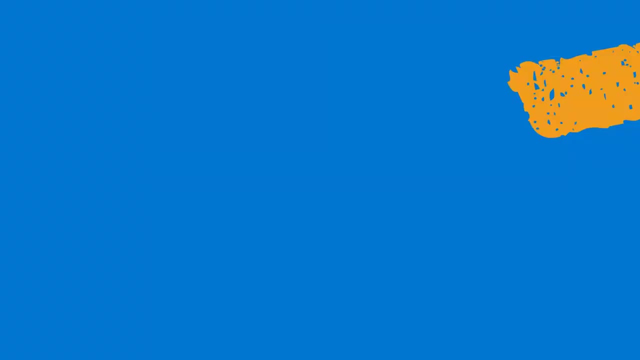 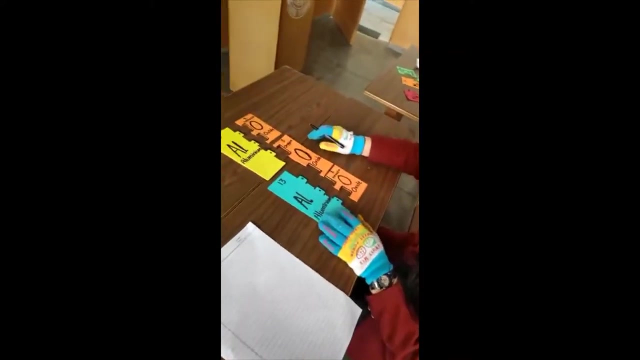 a card having three arms when combines with another card having one arm, so in this way we can join them in order to get formula of aluminum chloride as AlCl3, as three cards of chlorine are used here. yes, Malvika, what are you doing where aluminium has three arms and oxygen has two arms? 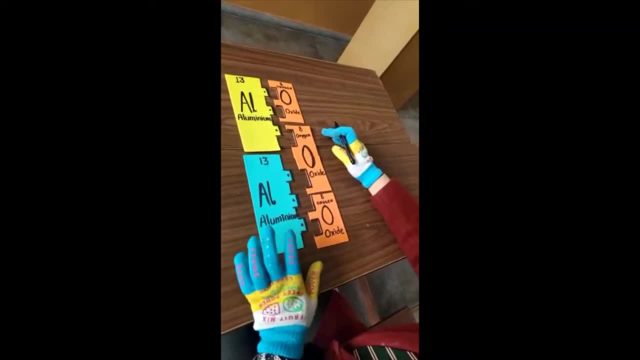 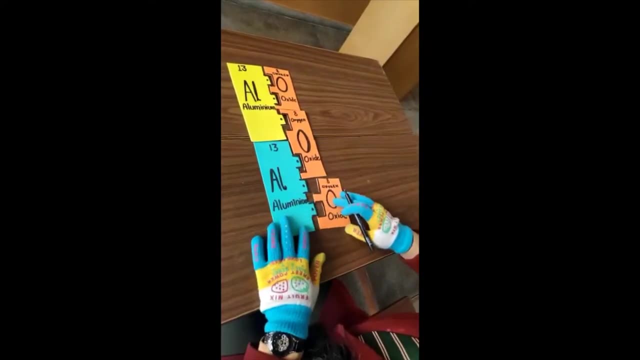 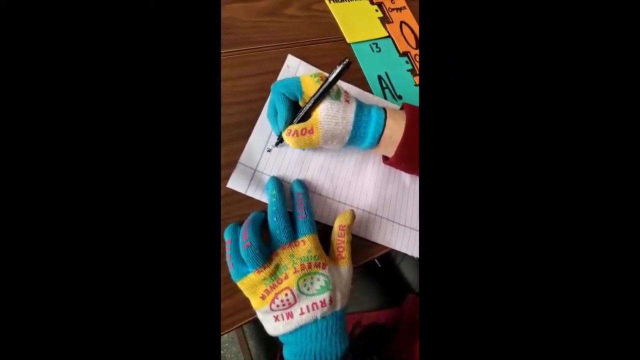 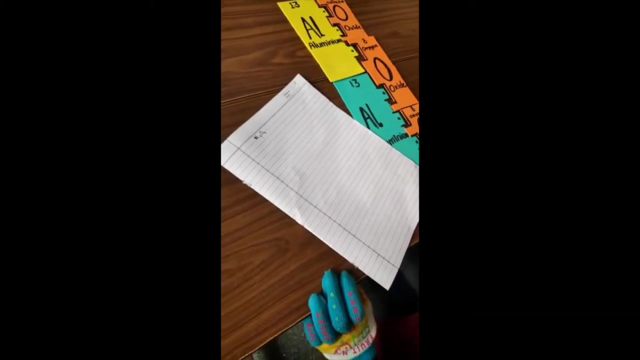 so to satisfy the property of aluminium oxide, we have taken two cards of aluminium and three cards of oxygen. when we combine these, it forms aluminium oxide. very good, can you write the formula? yes, ma'am, it is Al2O3. do you know how aluminium oxide is naturally found, ma'am, it is found in precious 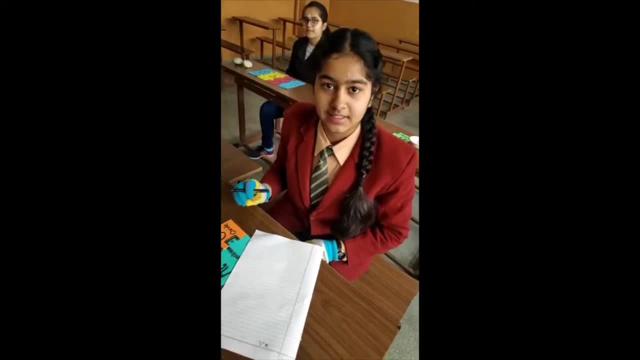 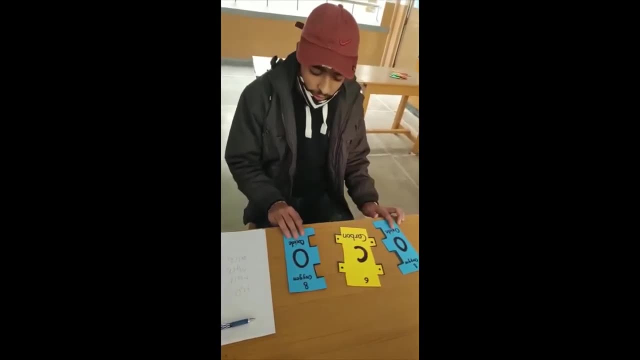 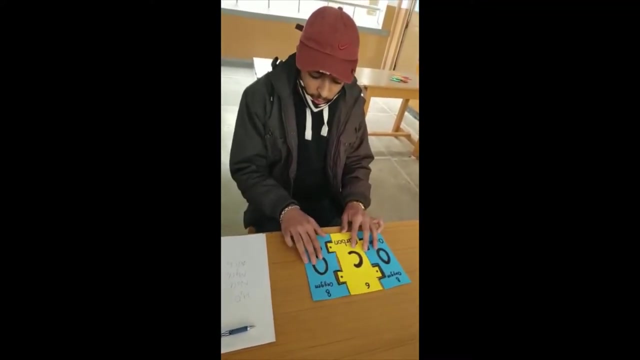 gels such as Ruby and sapphire. yes, very good. and, ma'am, I have also made a formula where carbon has valency 4 and oxygen has valency 4. carbon has four arms that can combine two oxygen atoms and forms CO2. it is the most common firm. 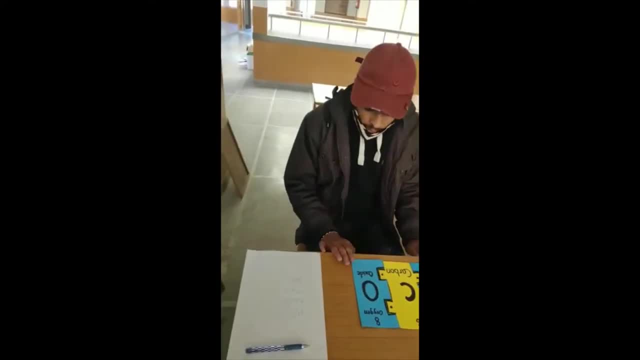 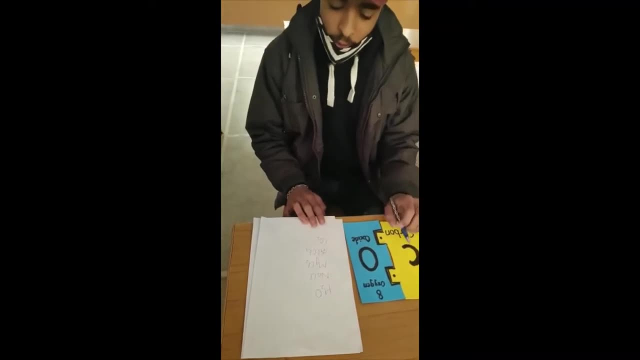 of a common gas present in the air. yes, very good. can you right the formula of hold dioxide connexion? it is CO2, yes, so yes, my heck, what you are doing. assme know that carbon has valency 4, so we can combine it with 3 oxygen atoms. so we can combine it with three oxygen atoms, sum to hold, but still everything is material金 ait safely, kaog WilAyat. 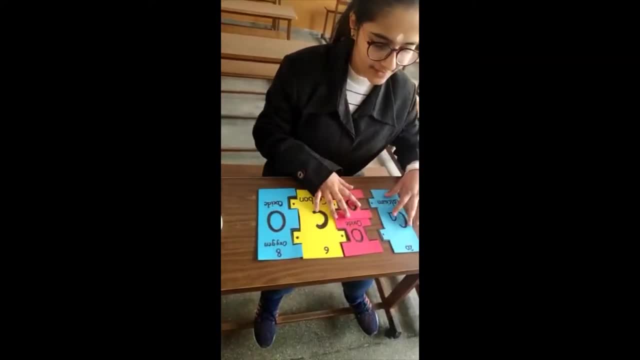 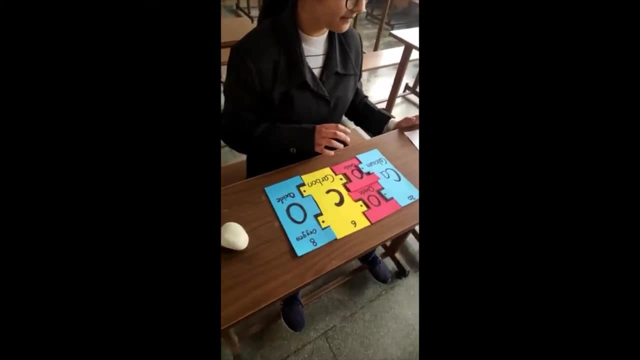 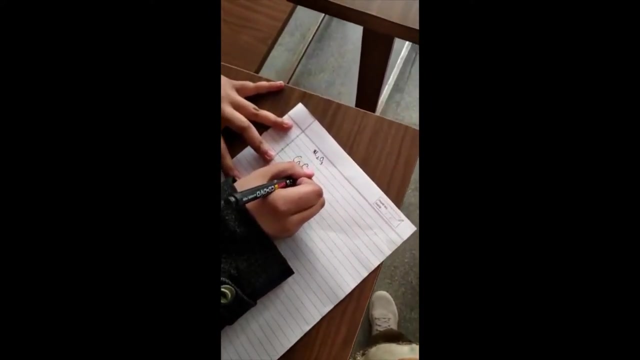 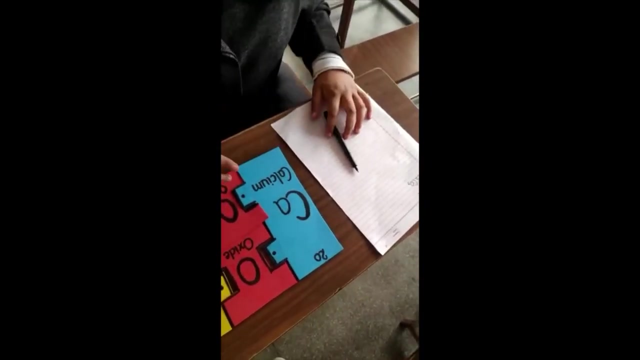 these two cards have their valencies left, So we can combine it with calcium that has valency 2 to form calcium carbonate- iron. Very good, Can you write its formula? Yes, ma'am, It is written as CACO3.. Very good, Do you know in what form? calcium carbonate? is available in our daily life, Ma'am. it is in the form of limestone, and even the marble on the floor is made up of CACO3.. Yes, Very good. So calcium carbonate is readily available in the form of limestone. Variety of limestone you can see around. Yes, Lavanya, Which formula. 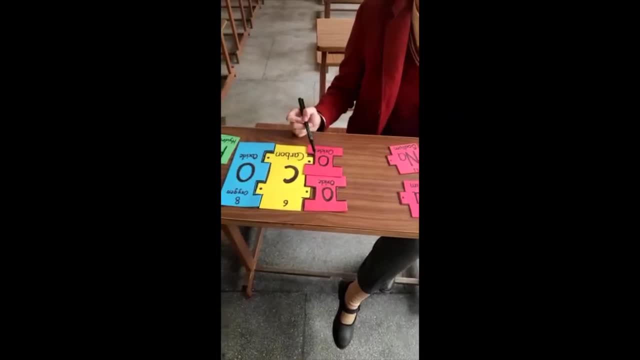 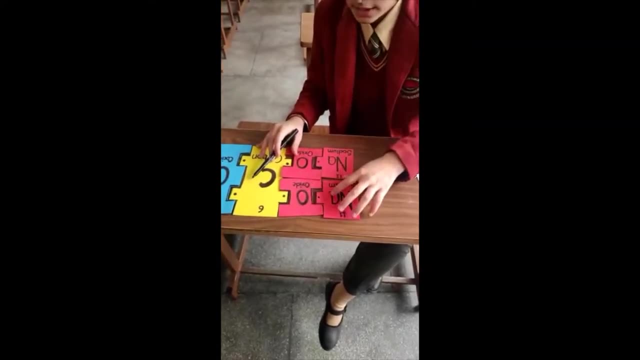 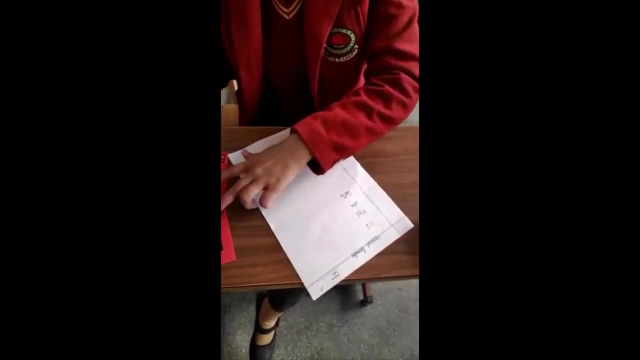 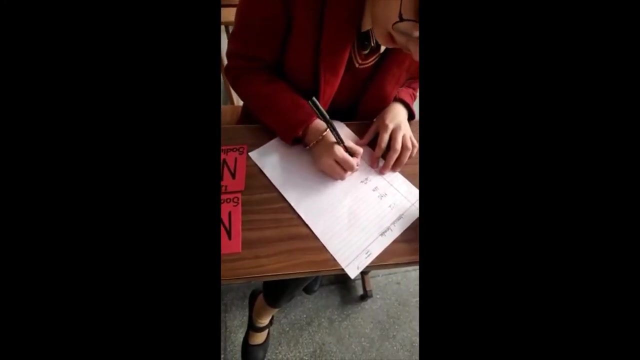 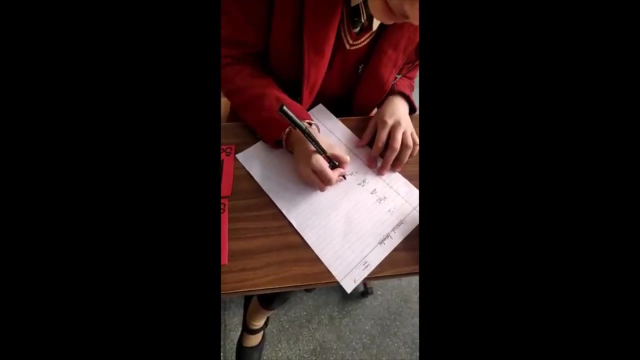 you have formed. This is CO3, carbonate iron, and if we join two sodium ions in this, it forms sodium carbonate. Can you write the formula of sodium carbonate? Yes, ma'am, As we have used two cards of sodium ion. we will write Na2 and this is the carbonate ion, so we will write CO3.. So the formula becomes: 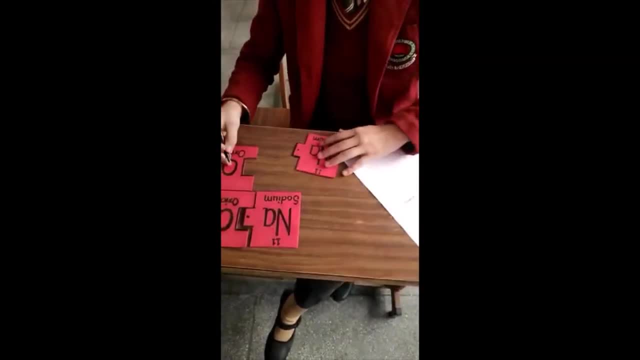 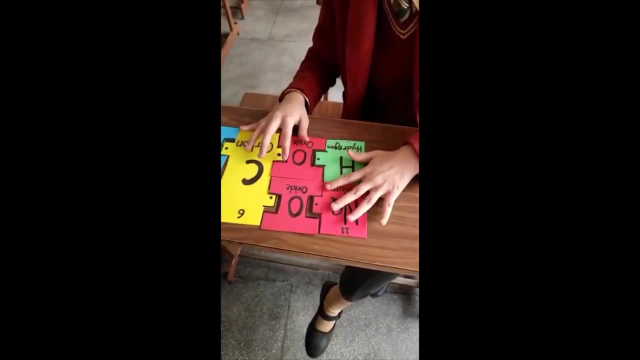 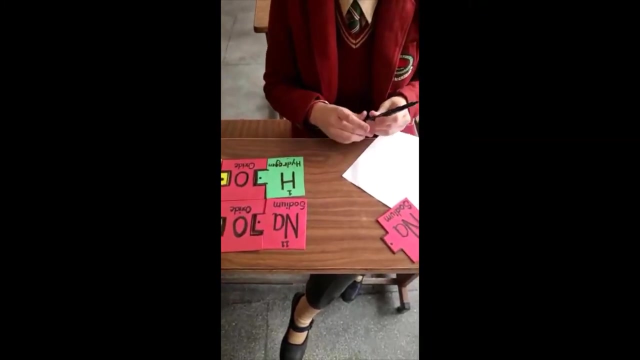 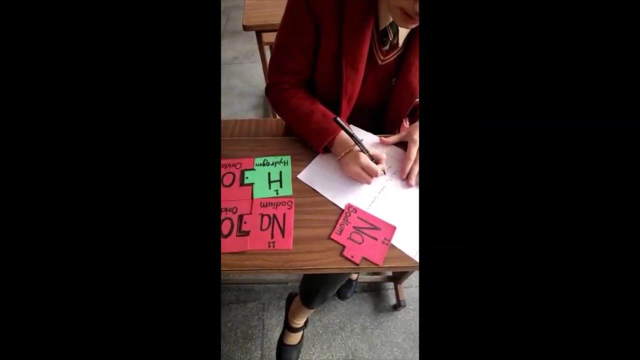 Na2CO3.. Very good, And if we take one hydrogen carbonate, we will write Na2CO3.. Yes, ma'am, And if we take one hydrogen ion, then this will become Na2CO3, which is sodium hydrogen carbonate. We will write it as Na2CO3.. This is commonly known as baking soda And you. 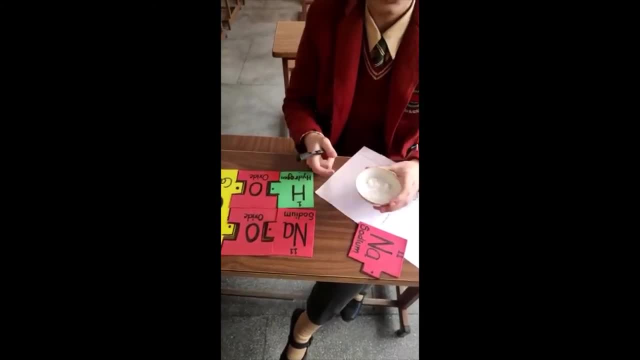 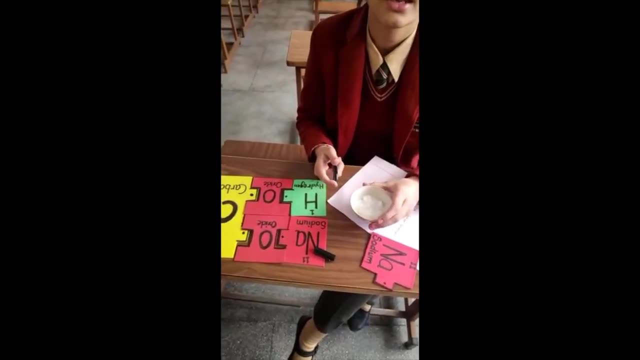 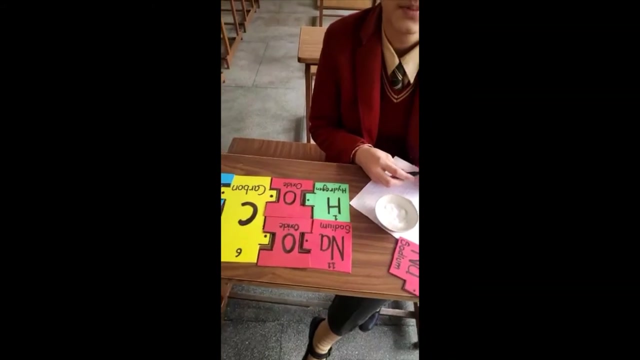 know baking soda is used in our kitchen also. Yes, ma'am, It is used in baking many things. It is used in cakes and idlis breads also- All these items in which fluffiness is required, where baking soda is added. Good Lavanya Bhumi, do you understand now why? sodium chloride? 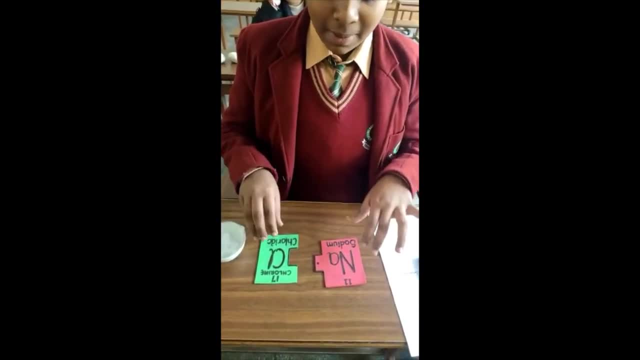 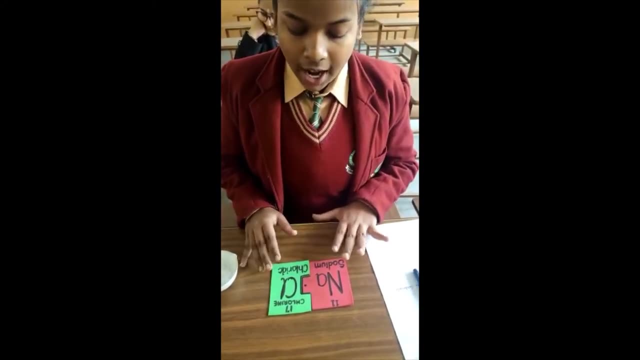 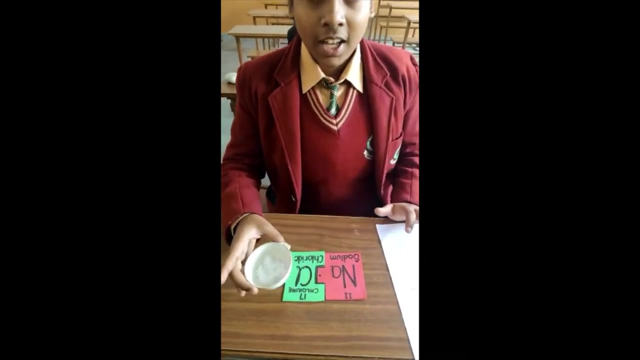 is NaCl not NaCl2?? Yes, ma'am, I have understood that sodium can combine with only one ion of sodium chloride and it forms sodium chloride And it is commonly used in our kitchen as a common salt. Very good.